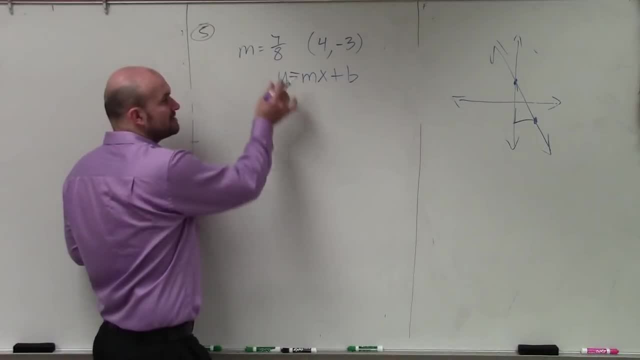 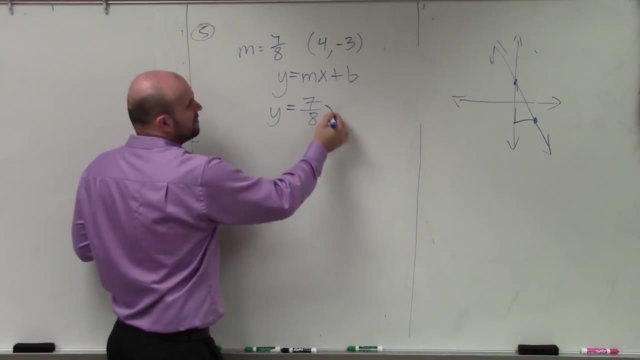 the slope and the y-intercept. Now, fortunately for us, this problem already gives us the slope, so that's easy. I can easily plug that into my formula. The problem is, though, we need to identify the y-intercept, And some students will make the mistake and say: well, 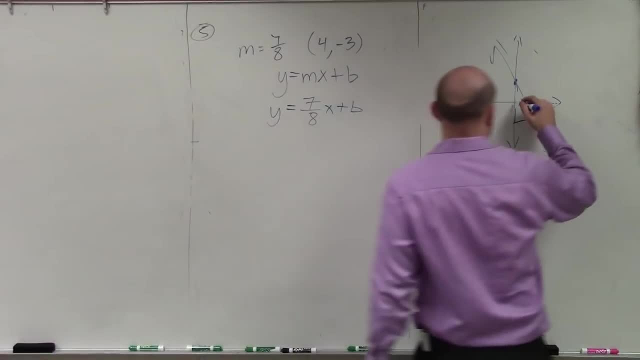 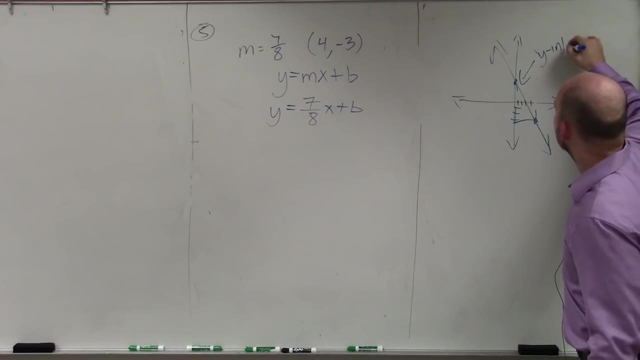 isn't this the y-intercept? No, this point is 1, 2, 3, 4, negative: 3, 1, 2, 3.. This point is over here. The y-intercept is right here. So, the important thing, the thing I want you. 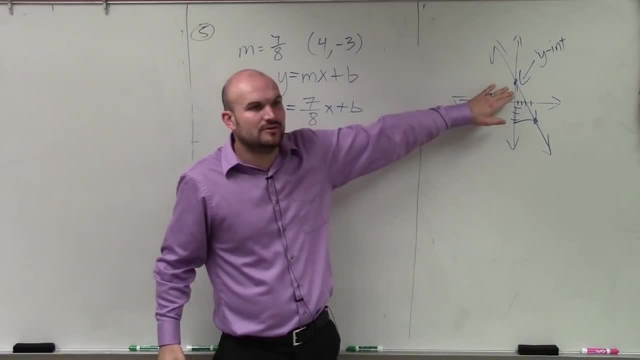 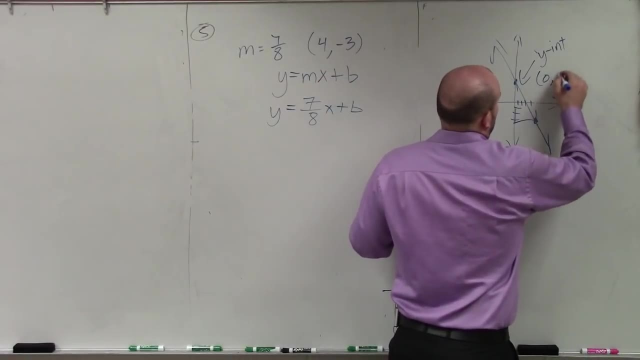 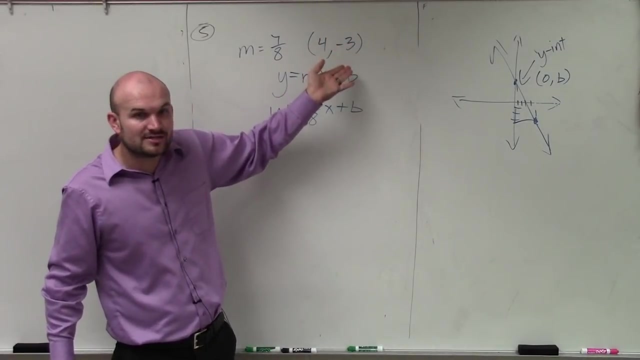 guys to understand is: what is the x-value at the y-intercept? What is the x-value at that point? Zero, Zero, Unless you have a point that's like 0 comma something. this is not the y-intercept, This. 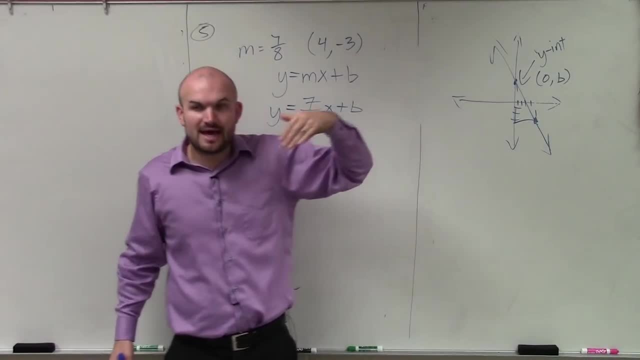 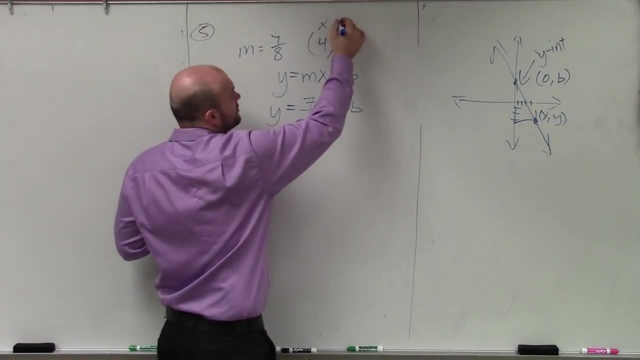 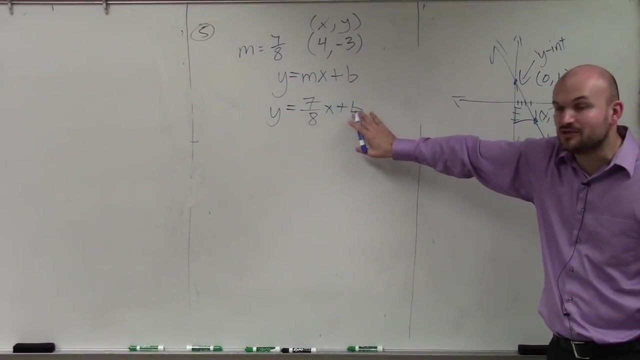 is just a point on the line, all right. And if it's a point on the line, that means it has x and y coordinates, all right. So, therefore, this point you can represent as an x, comma, y, Now to go ahead and solve for that, now to go ahead and identify, to find your y. 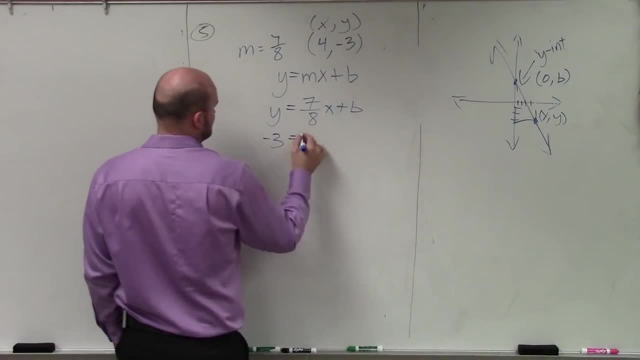 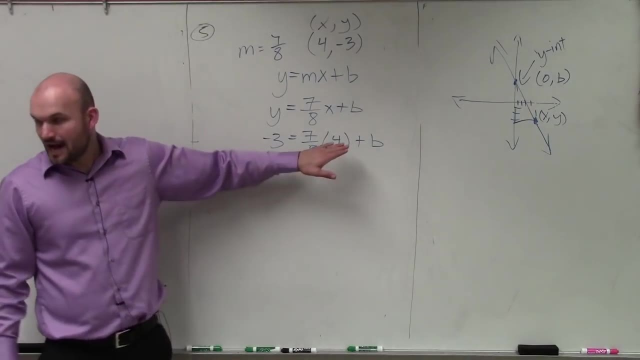 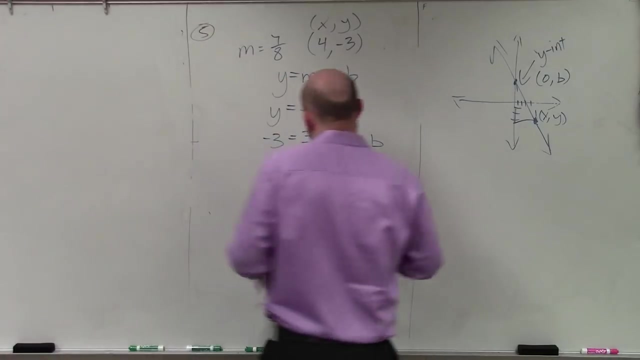 what we're simply going to do is plug in our x and our y coordinates. All right, Now again, how do we multiply? John, could you look over here for this, Because I'm kind of doing this for you. If you look at this, we're going to multiply a whole number. 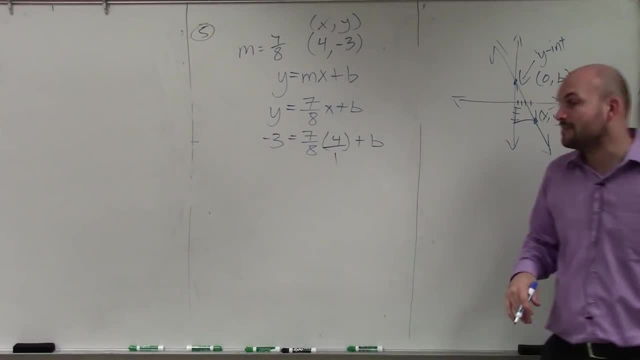 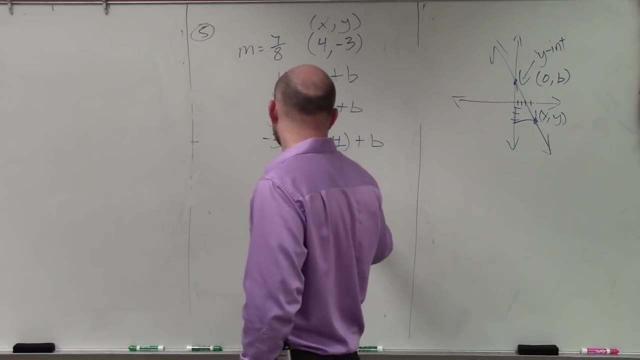 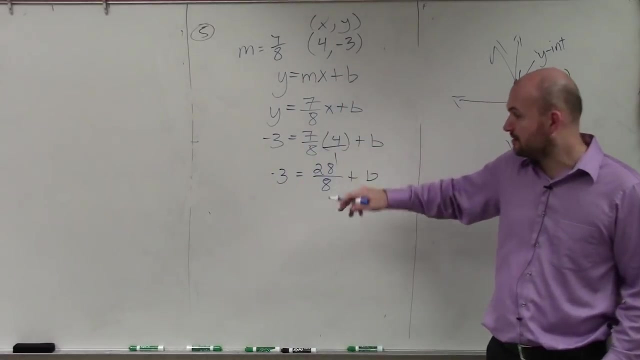 times a fraction. You convert the whole number to a fraction. Remember now we're multiplying two fractions. Excuse me, you multiply directly across. So I have negative. 3 equals 28 over 8 plus b. You could have simplified that. 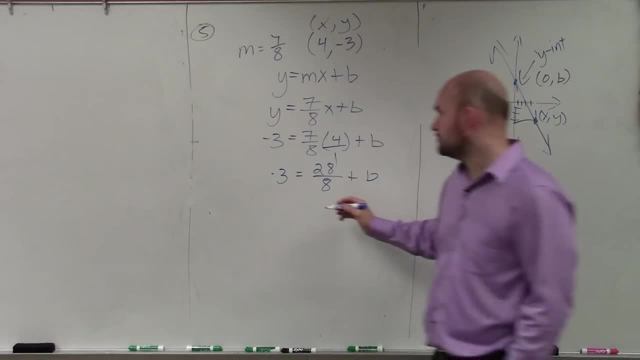 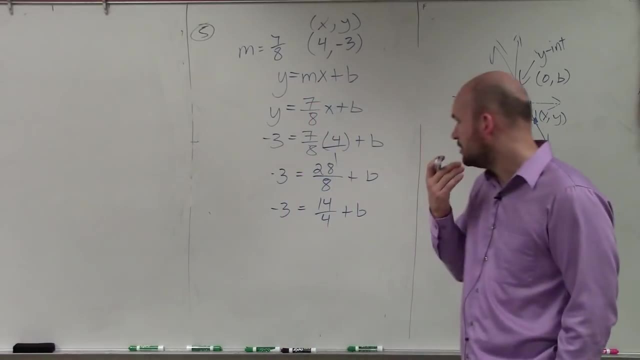 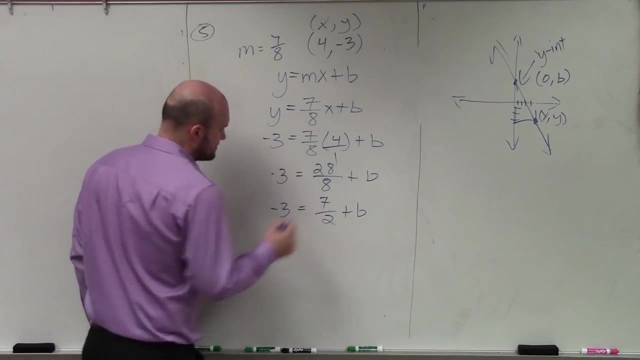 All right, Obviously, we can reduce this right to negative. 3 equals 14 over 4.. Oops, now I can reduce that even further. Let's divide by 4, right, 7 halves, which I could have done right up. 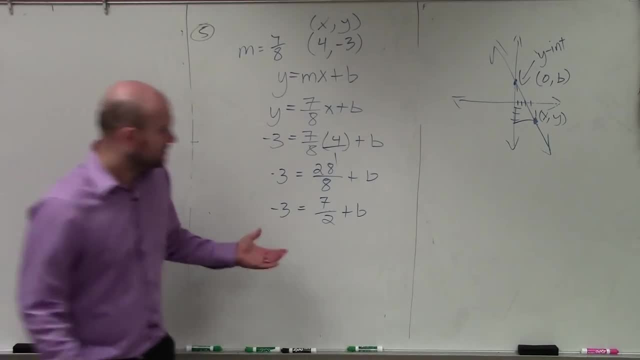 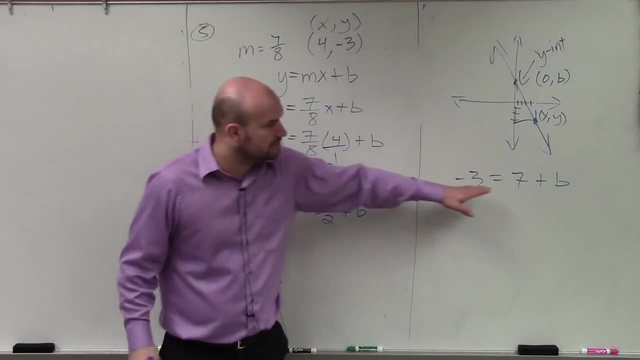 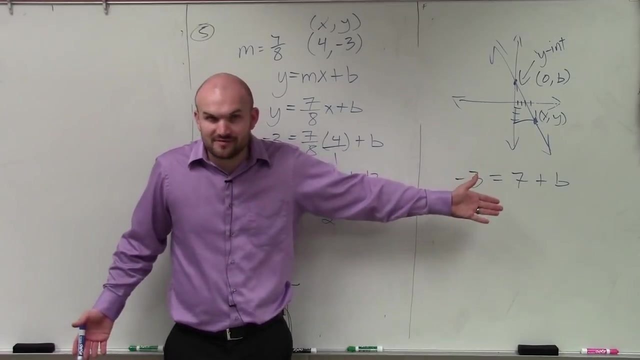 there. So let's reduce it down to 7 halves. Now this was getting me a lot. I was having trouble with students doing this. If I had that equation, this equation, right here, what would I do to solve for b, Subtract 7,, right Is everybody? 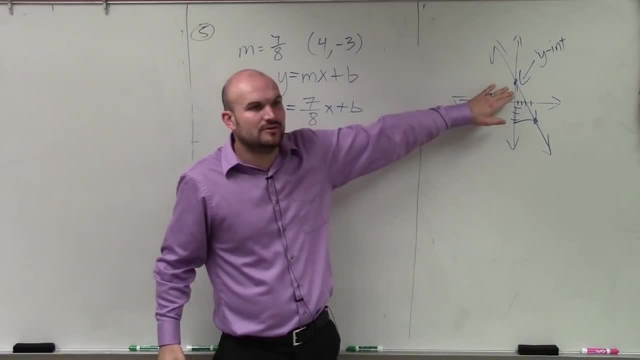 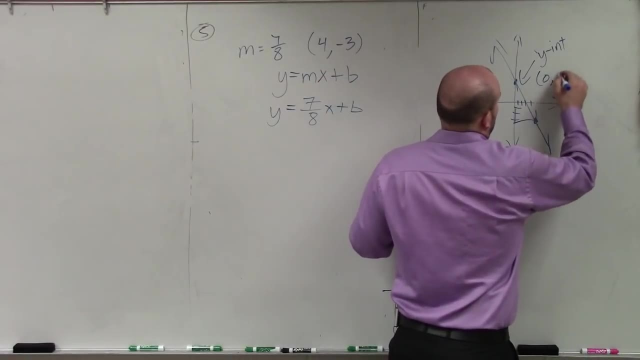 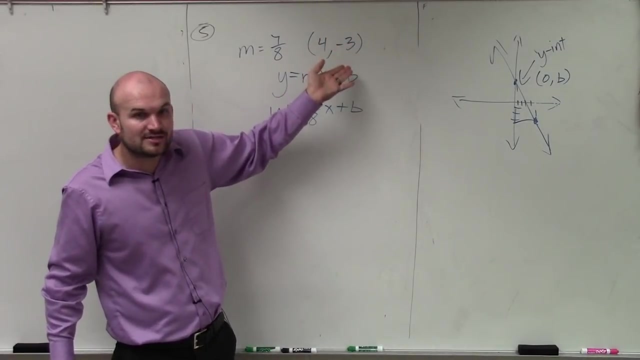 guys to understand is: what is the x-value at the y-intercept? What is the x-value at that point? Zero, Zero, Unless you have a point that's like 0 comma something. this is not the y-intercept, This. 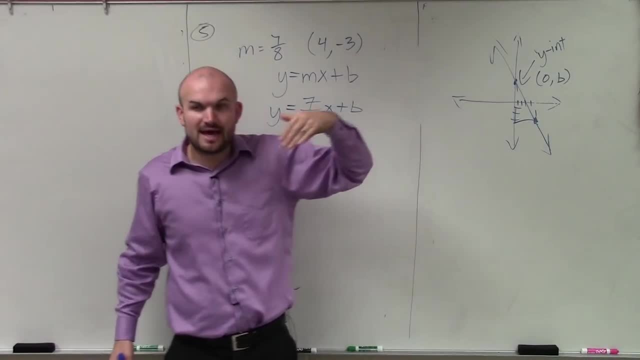 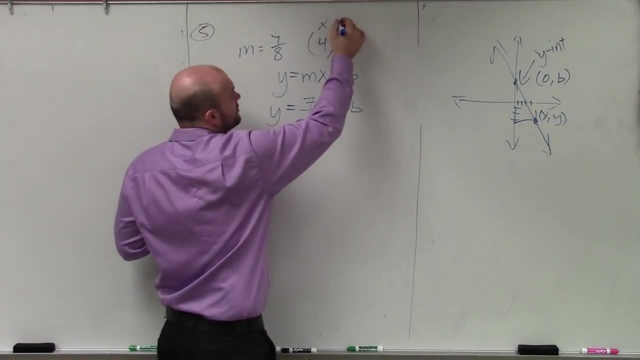 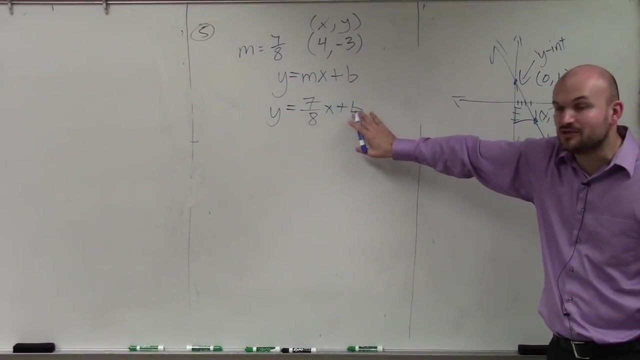 is just a point on the line, all right. And if it's a point on the line, that means it has x and y coordinates, all right. So, therefore, this point you can represent as an x, comma, y, Now to go ahead and solve for that, now to go ahead and identify, to find your y. 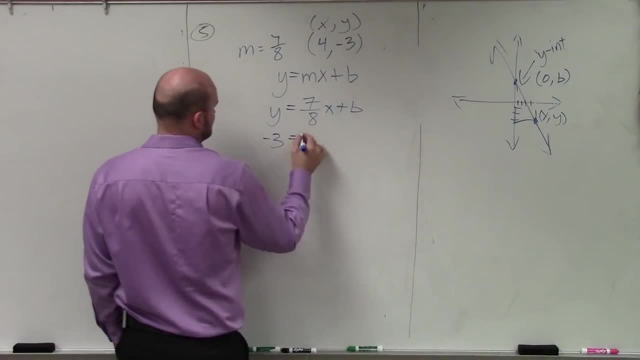 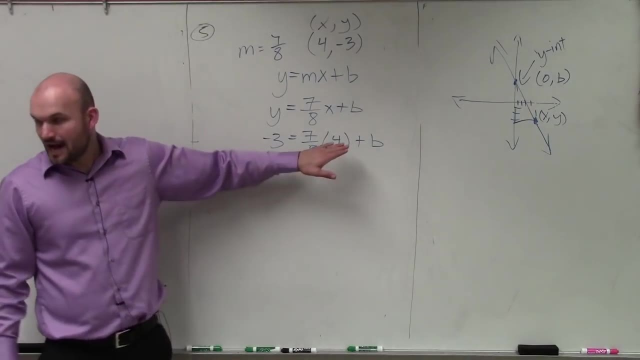 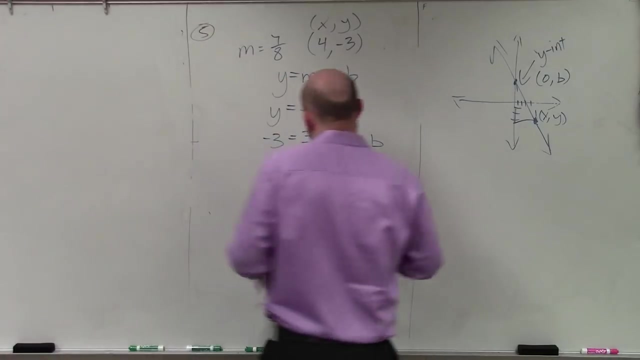 what we're simply going to do is plug in our x and our y coordinates. All right, Now again, how do we multiply? John, could you look over here for this, Because I'm kind of doing this for you. If you look at this, we're going to multiply a whole number. 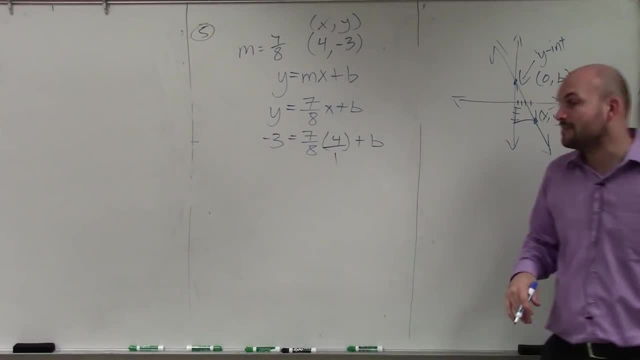 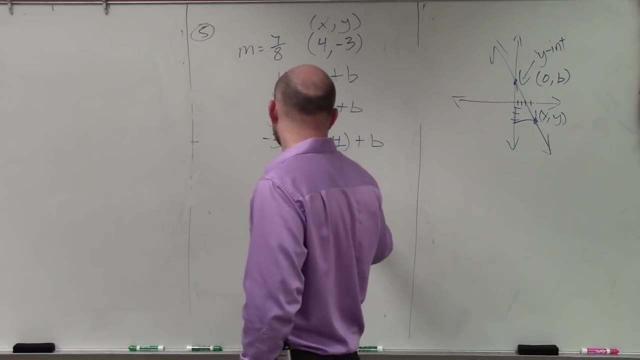 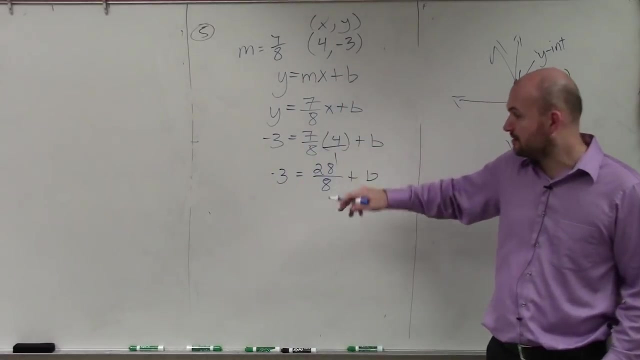 times a fraction. You convert the whole number to a fraction. Remember now we're multiplying two fractions. Excuse me, you multiply directly across. So I have negative. 3 equals 28 over 8 plus b. You could have simplified that. 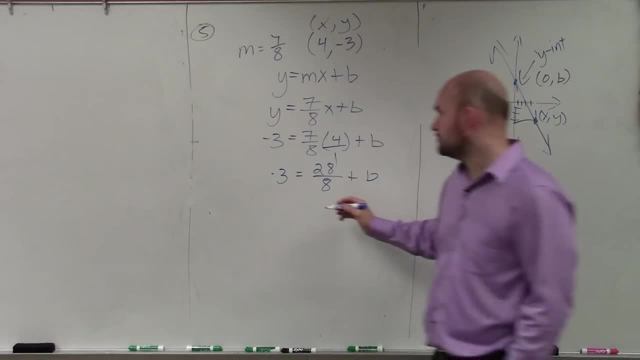 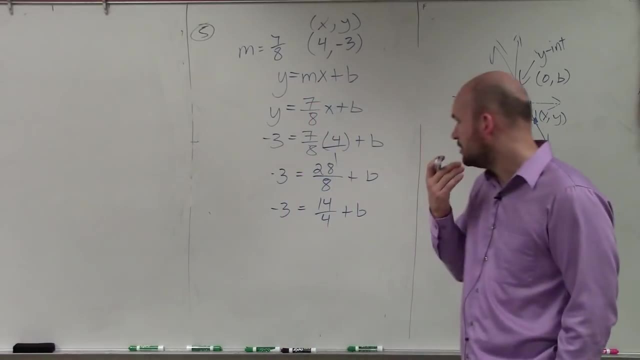 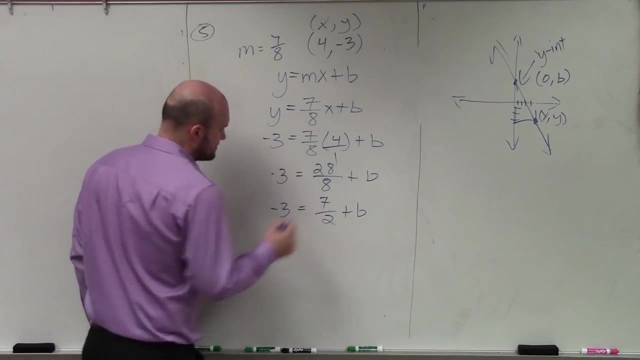 All right, Obviously, we can reduce this right to negative. 3 equals 14 over 4.. Oops, now I can reduce that even further. Let's divide by 4, right, 7 halves, which I could have done right up. 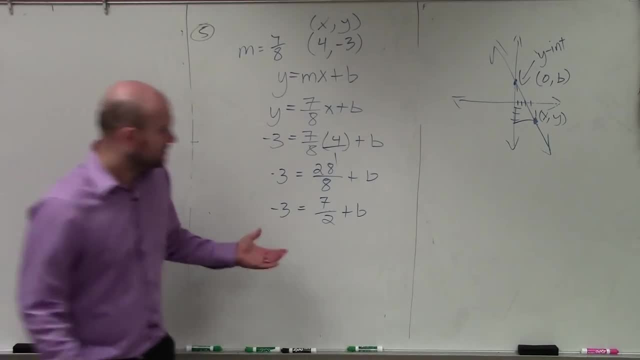 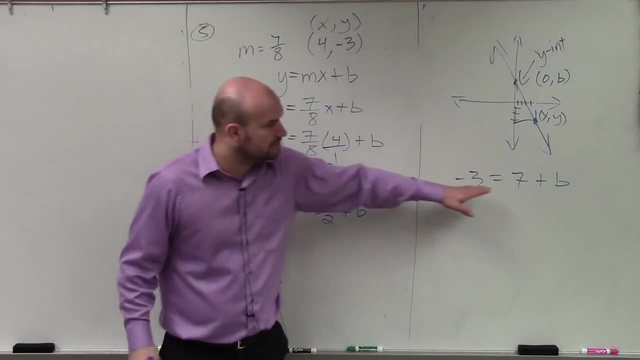 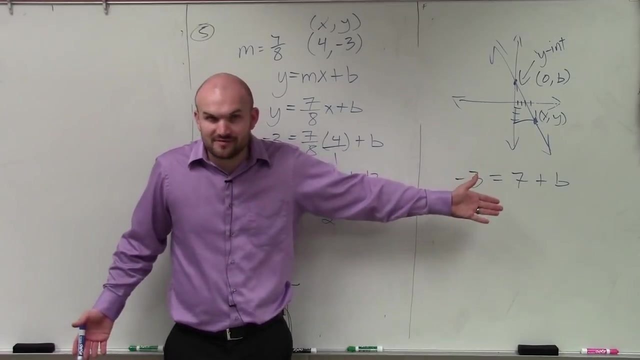 there. So let's reduce it down to 7 halves. Now this was getting me a lot. I was having trouble with students doing this. If I had that equation, this equation, right here, what would I do to solve for b, Subtract 7,, right Is everybody? 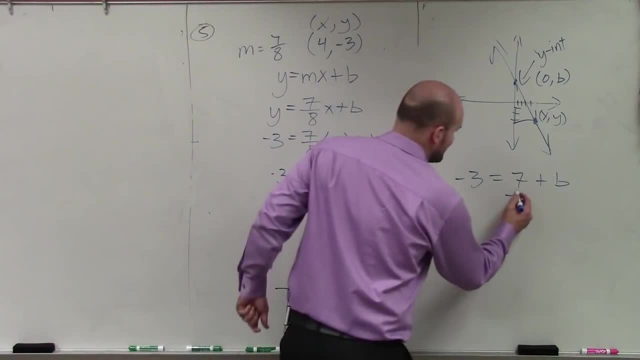 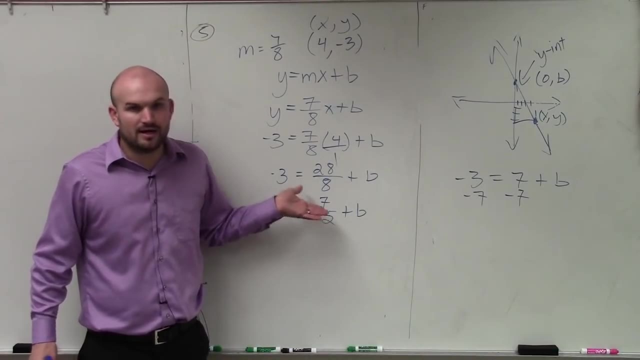 okay with me on that one, Everybody was with me. Subtract 7. You get the b by itself. So, ladies and gentlemen, it amazes me. Just because this is a fraction, people say, oh, I don't know what to do. It's the same thing. 7 or 7 halves. This is a number, That's a number. 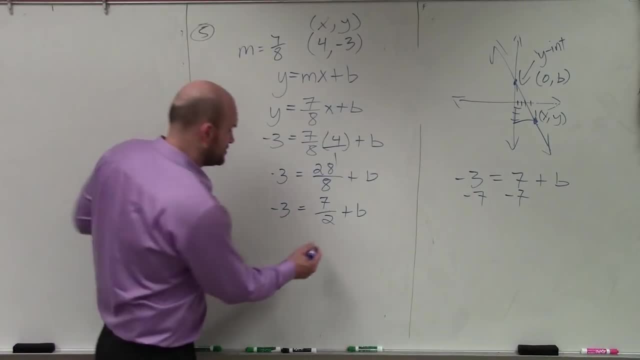 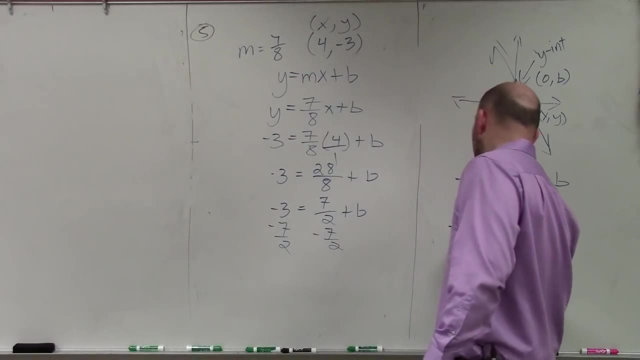 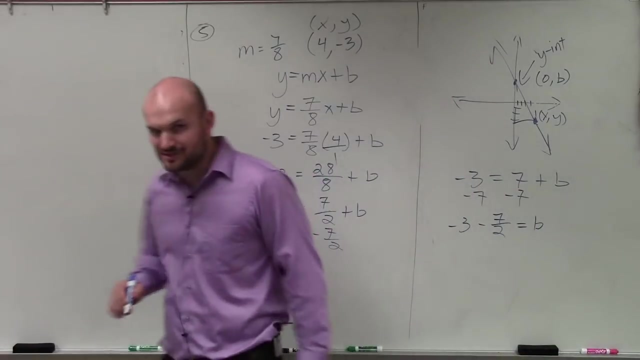 This is just a fraction, So you subtract 7 halves On both sides. So now I have negative 3 minus 7 halves, And I know why you don't want to know what to do, because you do not want to be subtracting fractions. But basically when